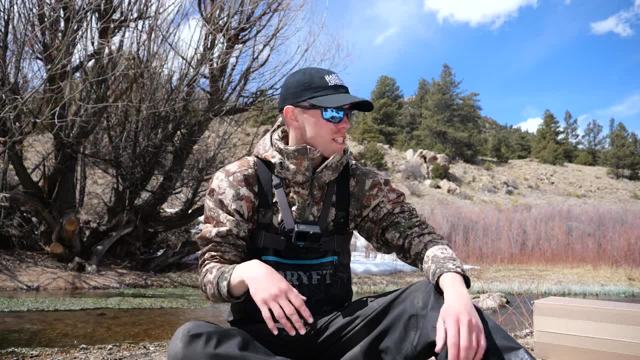 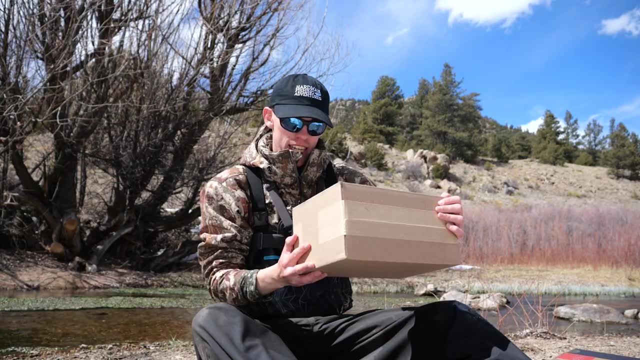 You only pay for what you want. Alright, guys. so hopefully the wind kind of stays calm for us. I'm going to show you guys two boxes here I've got. I'm going to start off with the trail kit. This is the trail box. 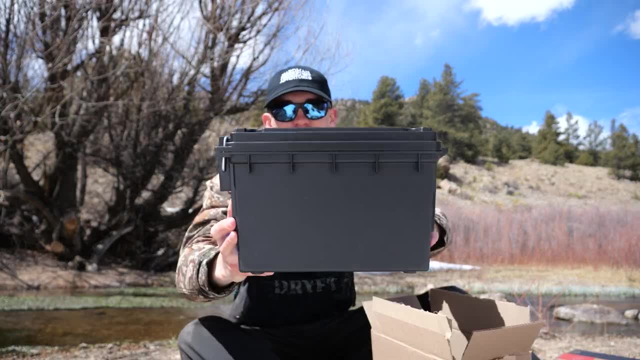 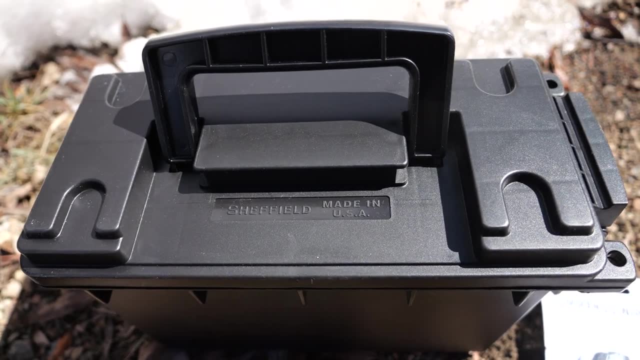 Here we go. Look at this. I think it all comes in this nice little, nice little crate here And this is a field box here and we're going to open this up. This is a really kind of nice. Honestly, Our first item in here is Surviving the Great Outdoors. 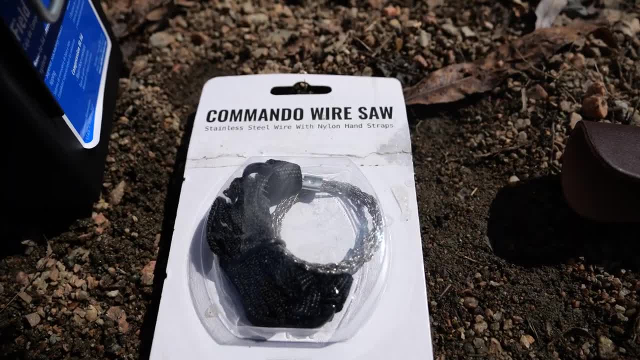 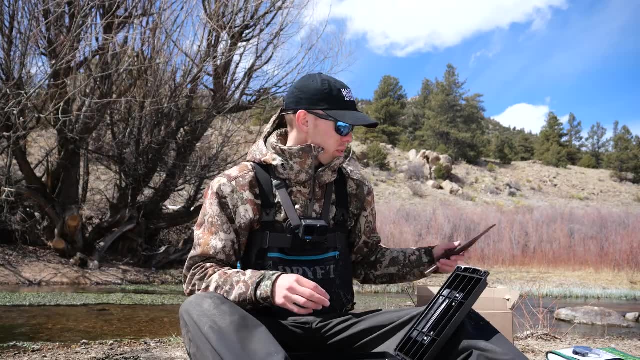 We have a paracord bracelet here. a wire saw. This is the knife that it comes with. The brand is R I L L Trail Simple Tools. That's the first box, though Let's get into the second box. Oh, here we have a nice card that shows what is in the box. 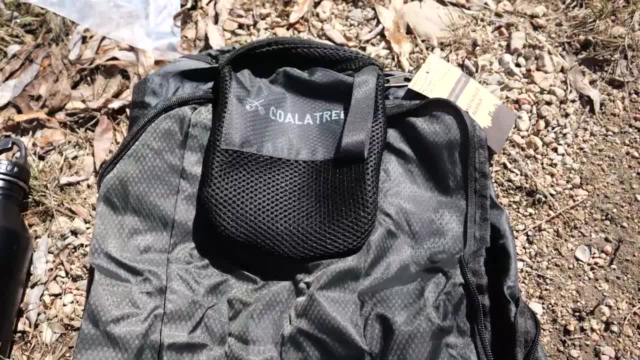 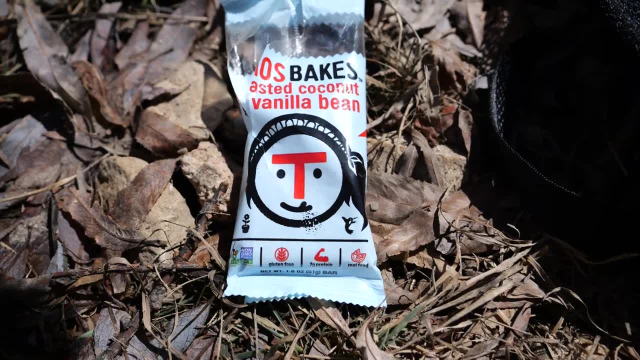 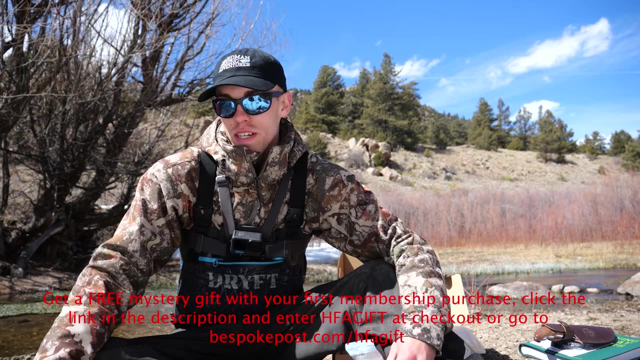 So here we have the Nomad packable backpack, an M8 water bottle, survival LED headlamp and a toasted coconut plus vanilla bean bar. All right, Well, thanks to Bespoke Post for sponsoring this video To get yourself a free mystery gift with your first membership, you can. 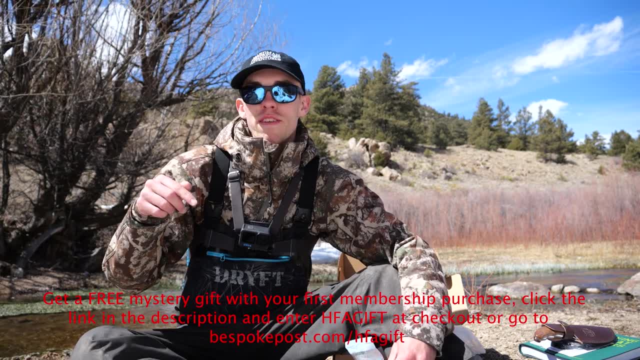 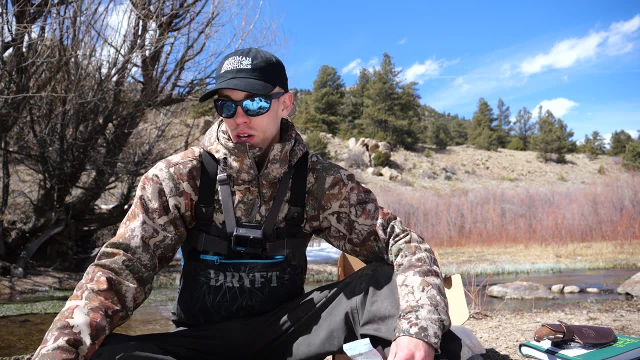 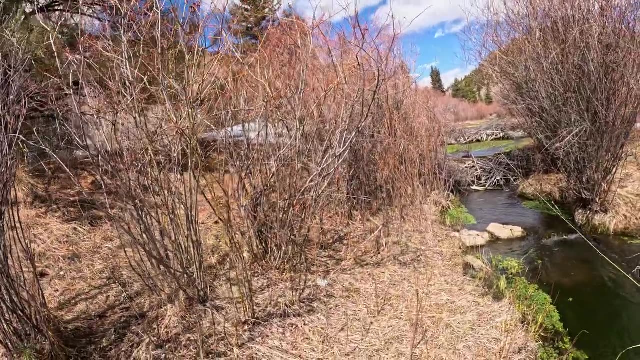 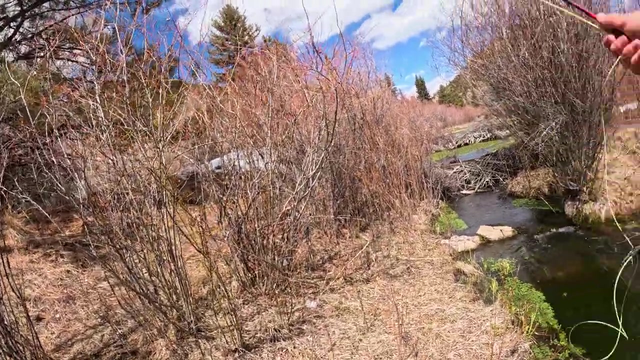 go to the link in the description and check out, enter in code: HFA gift or you can go to bespokepostcom forward, slash HFA gift, which I will have linked down below as well, And let's get back into the fishing. You got a big fish, got him. 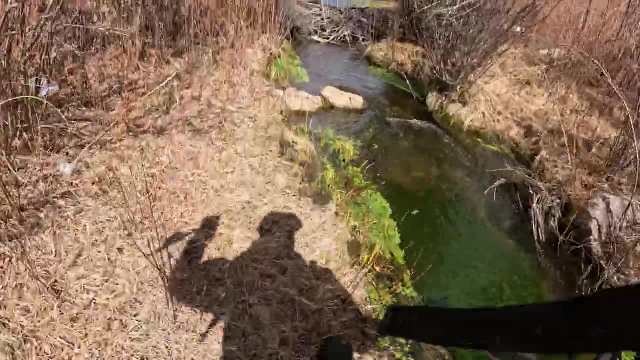 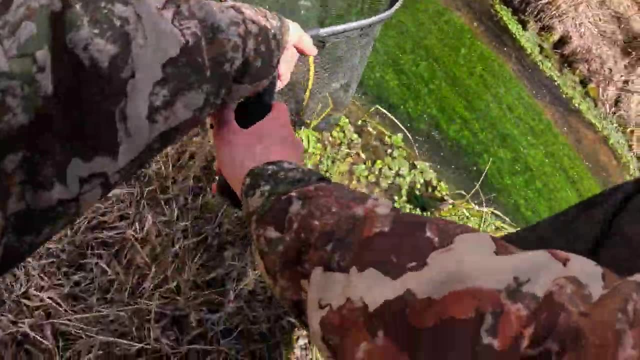 It is a giant. Oh my gosh, He's in the weeds. Well, that'll work. I couldn't tell if that was a fish or not, but it was. Oh my gosh, Another nice, nice little brown trout right there. 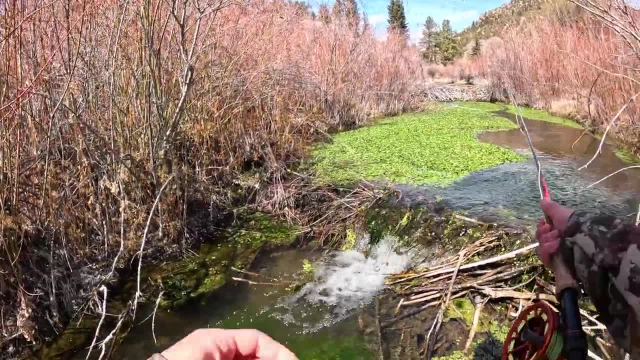 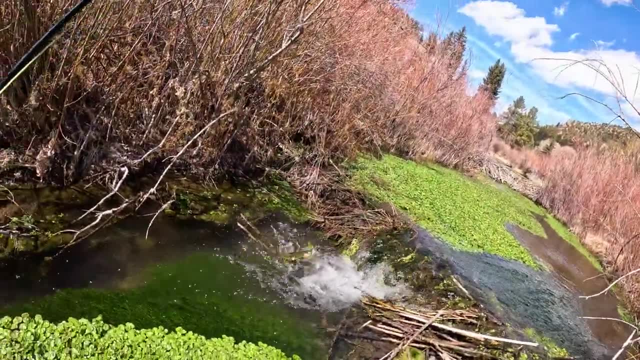 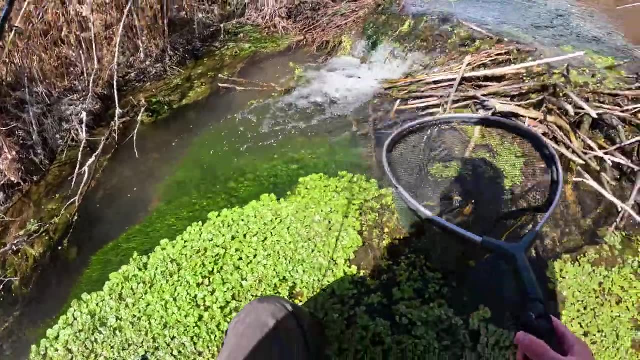 Here, bud, you know I got him. Oh, he jumped out of the water for it. I can't get my net. I'm stuck in 20 trees. Here we go. I jumped out of the water for it. I doubt you could see that, but he wanted it. 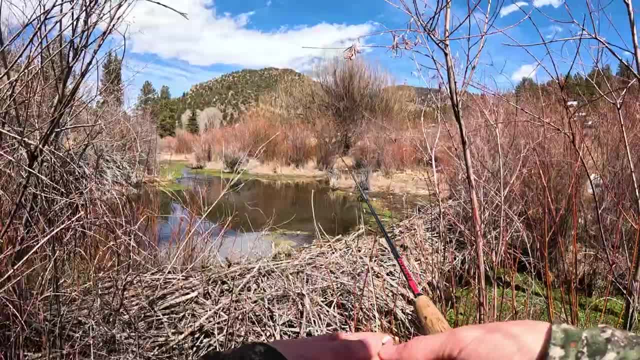 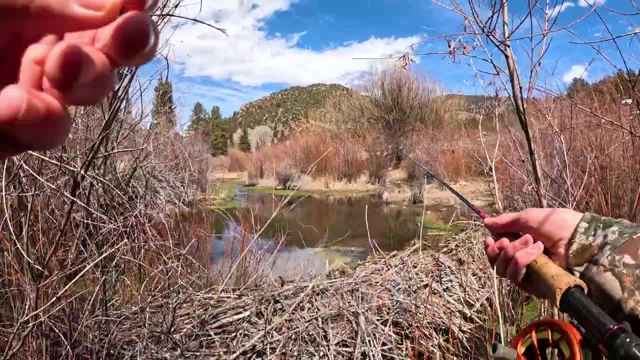 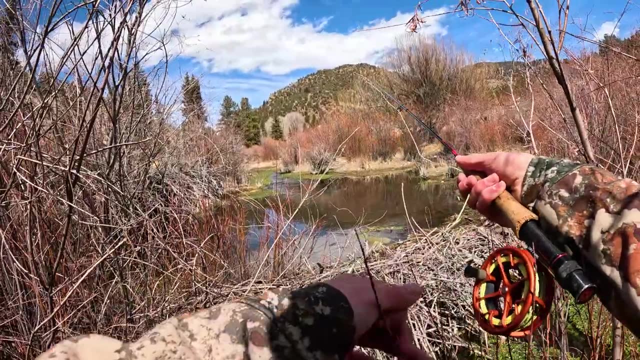 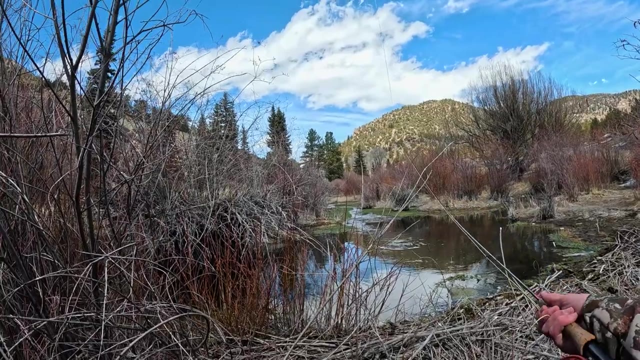 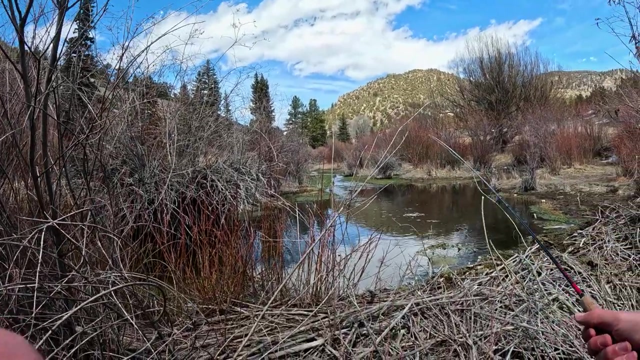 Little brownie. Let's get him back in that hole. 20,000 fish here, So I can't catch one of these. He's going to go home. That was the worst catch I've ever seen in my life. He didn't want it. 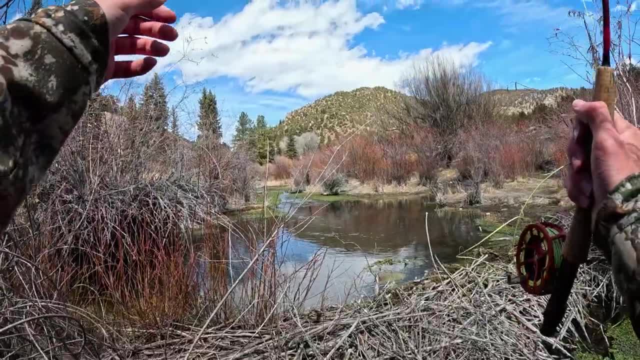 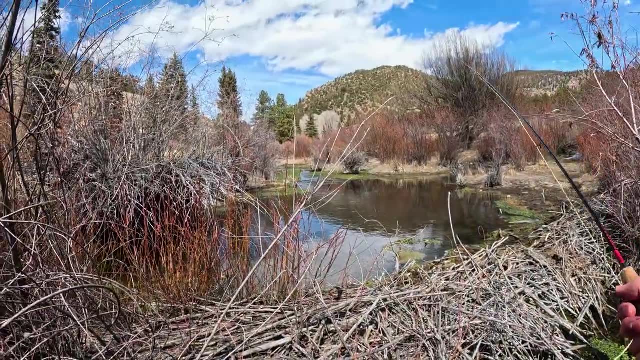 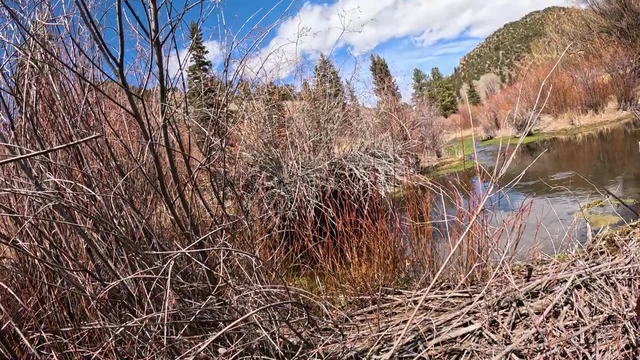 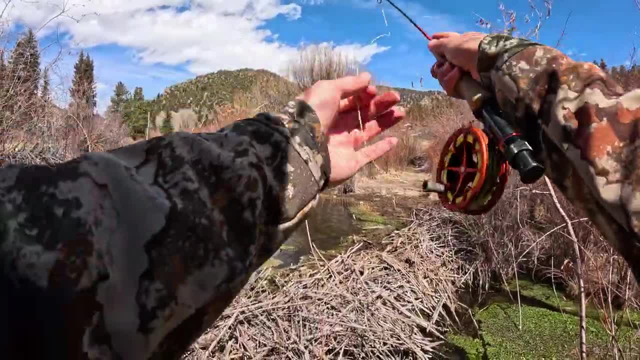 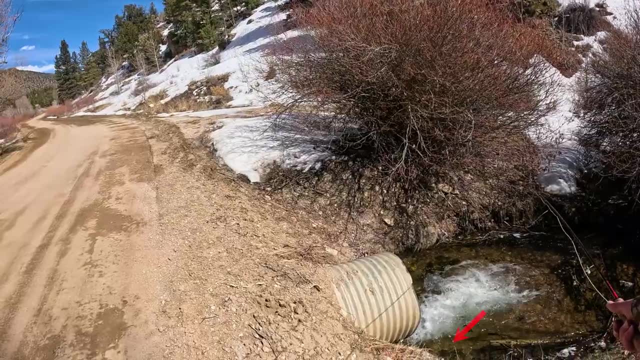 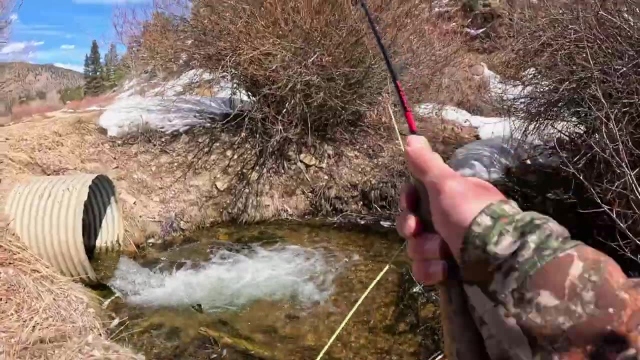 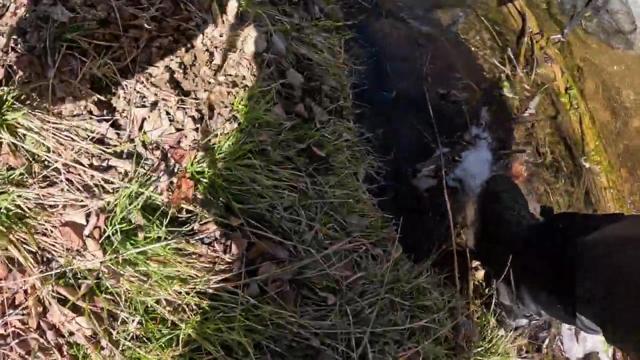 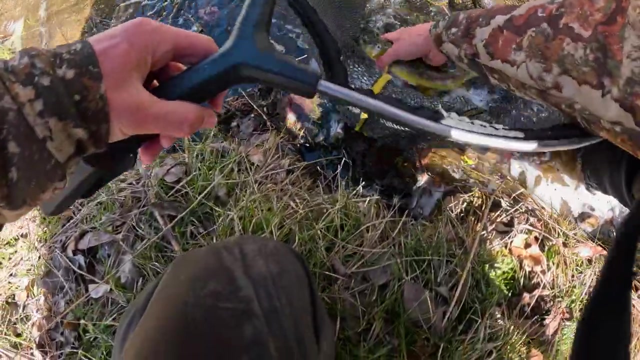 I give up. Just take me home, got him. oh, i didn't think that i was gonna see a fish. oh gosh, he's got me tangled. come on in here, buddy. you're tangled me up, there we go. i can't believe it. i can't believe it. he just came up and slurped it right up. 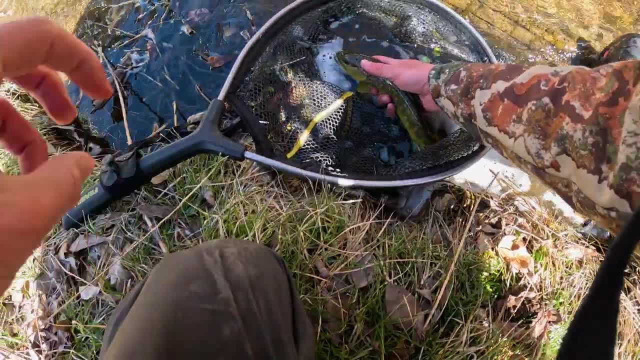 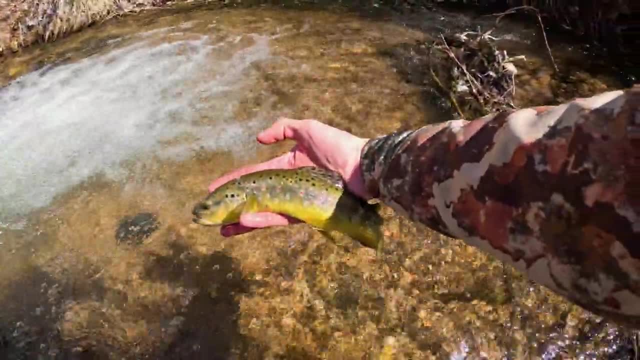 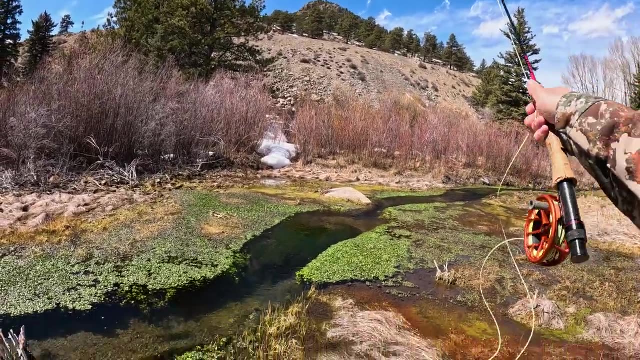 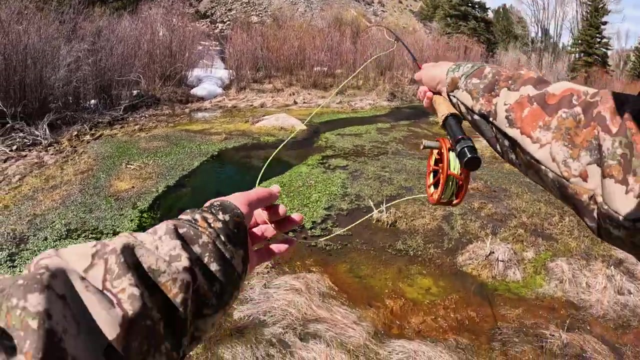 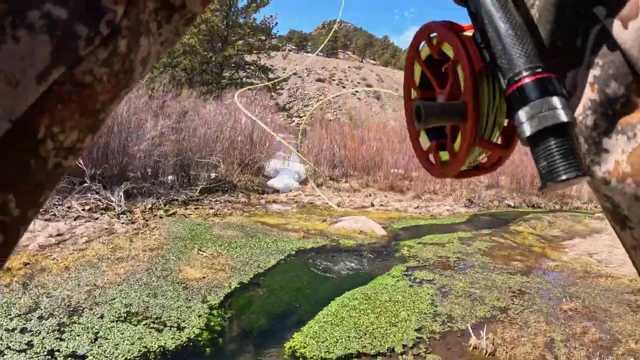 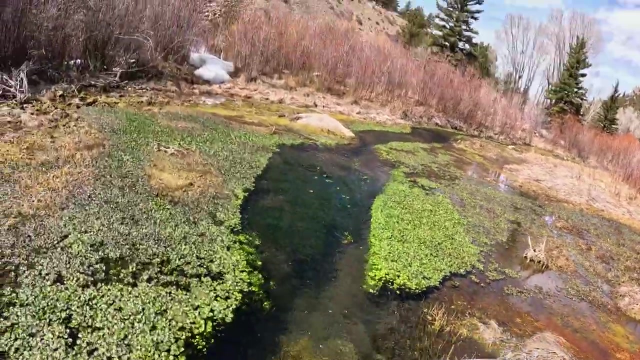 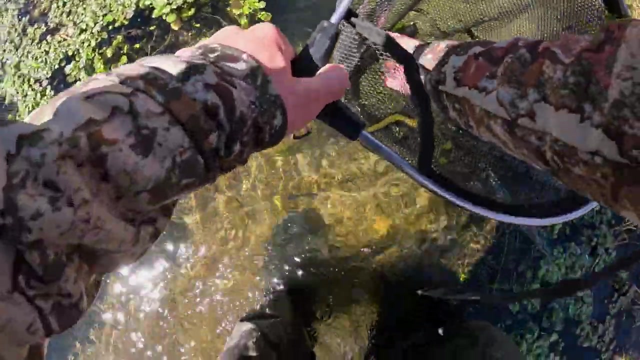 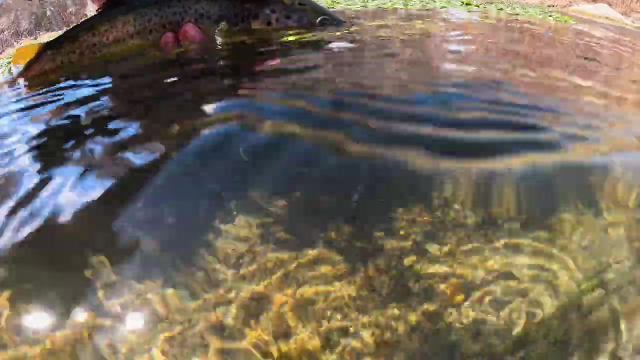 there we go, so easy to work. nice brown trout, pretty fish, that's a good one in here. buddy, good fish, come on down, got him. yes, back on it. it's a beautiful, that's it. that's the biggest fish, yet it's a good size, brown oh. 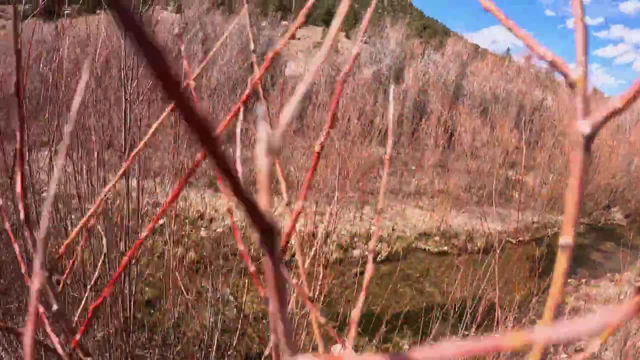 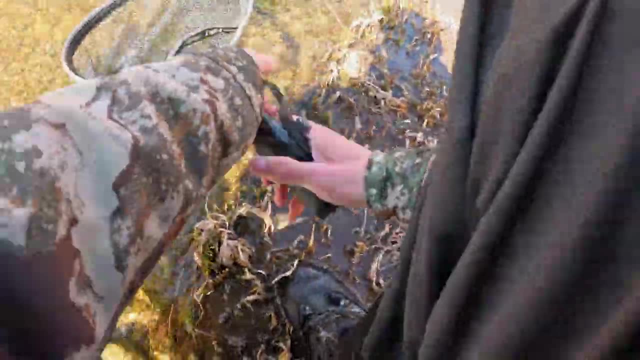 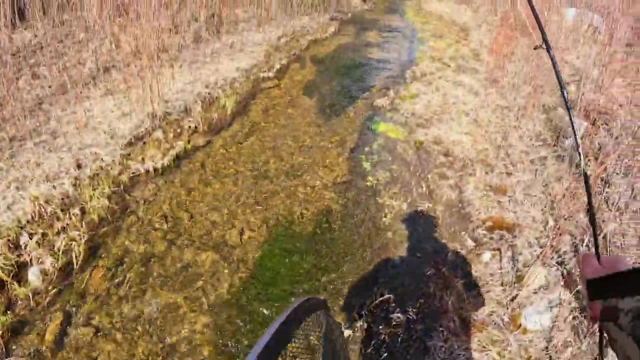 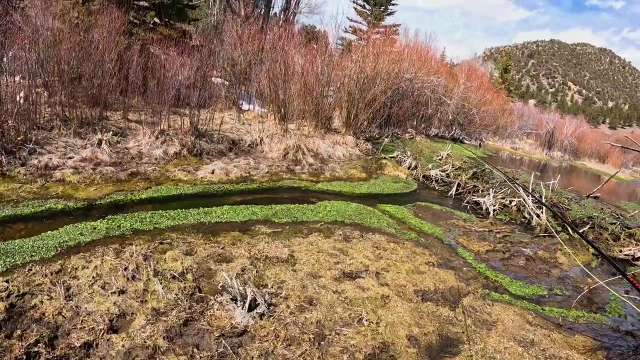 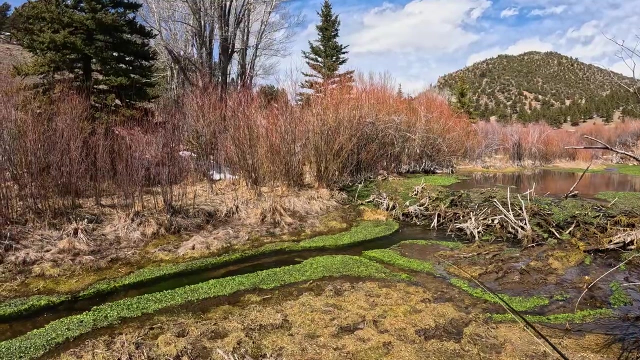 got him. no, let's not go in the in the trees. got him small guy, but still fish, definitely gonna be some more. up in here found a small elk or caddis. see if this is gonna work. it's smaller and the hook is, so on this I don't even hook anything, even if it does eat, but we're gonna give it a shot. 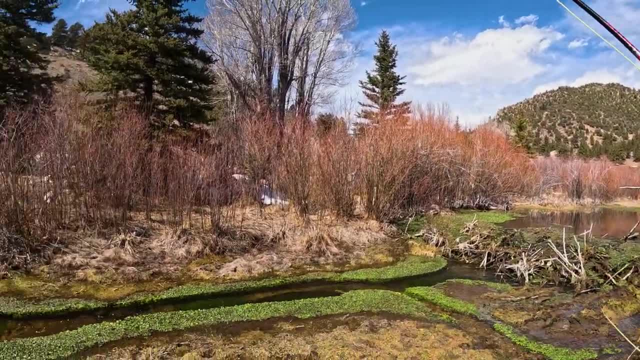 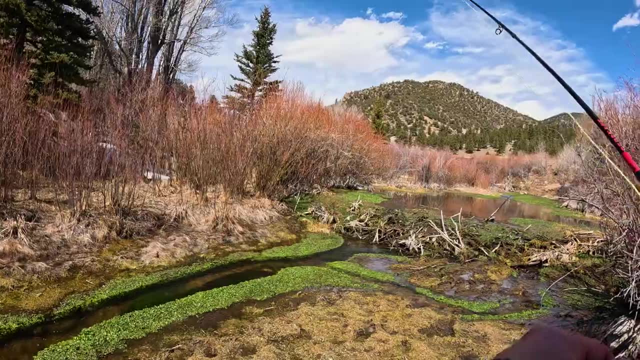 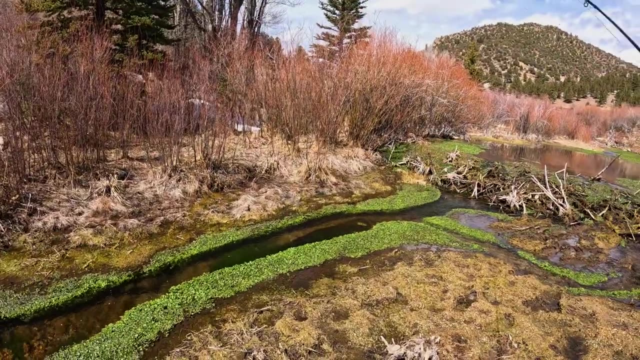 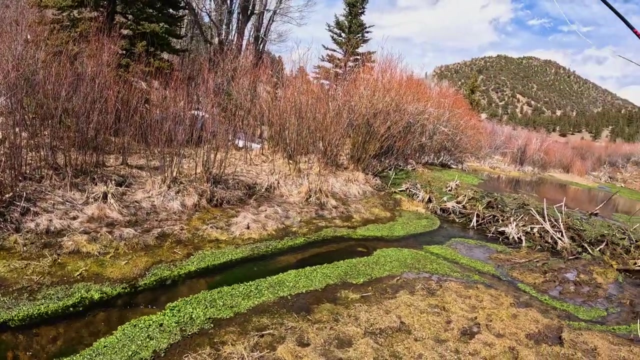 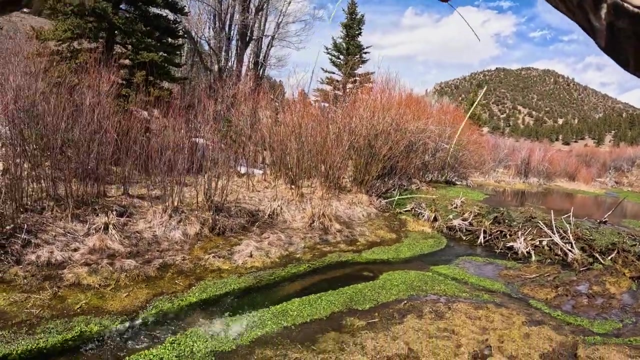 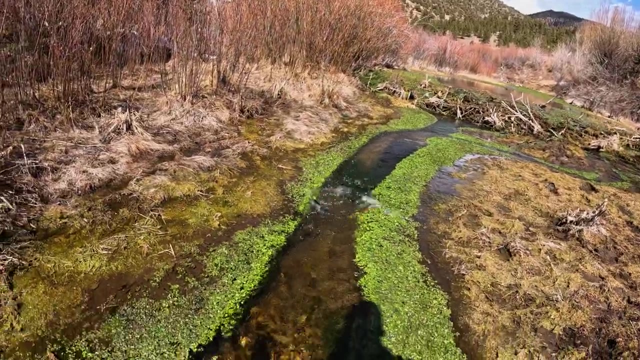 dang it. he would have eaten that for sure. I just my line is getting caught in every little piece. I guess not. he just didn't see it. it's a good one, just stay right here, stay on there, buddy, come back, come back to me. yes, he did eat it. 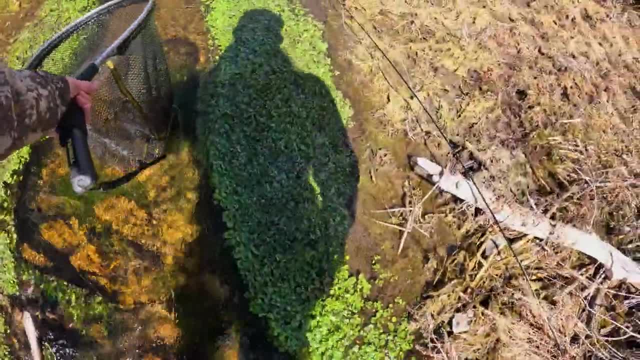 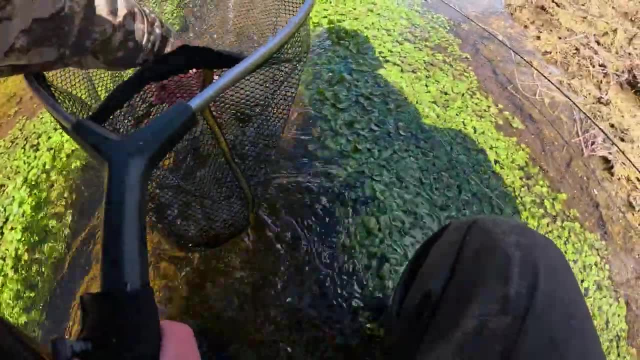 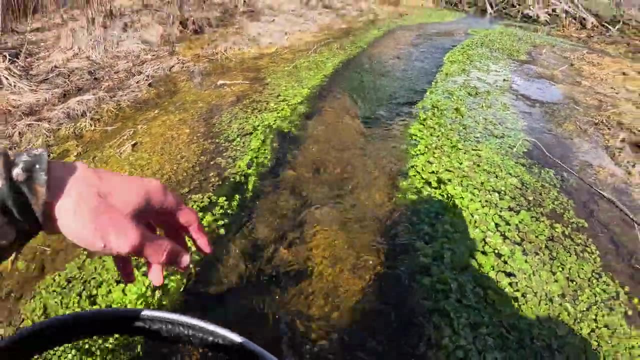 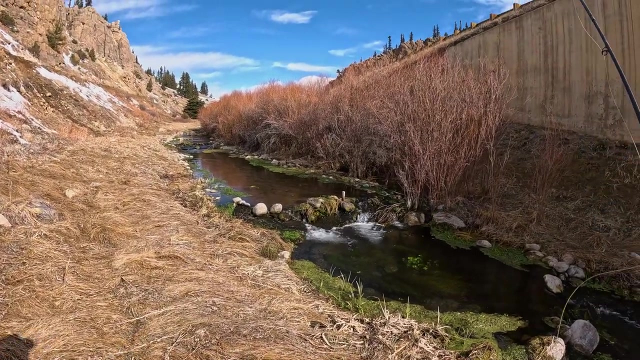 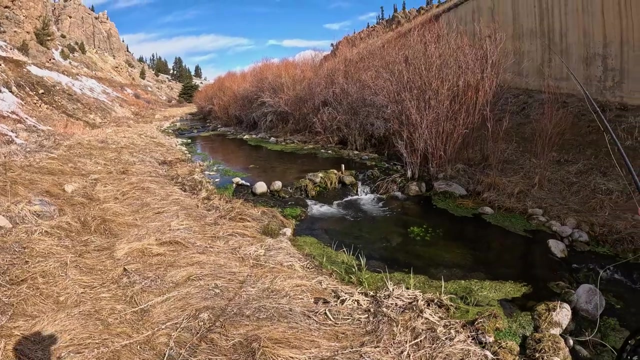 he was speeding. I thought he would, but he's just not happy. I guess with the first few times it's not a bad fish at all. there we are. this guy is so ready to go something funny. there we go. nice brown becky guys. oh a win. 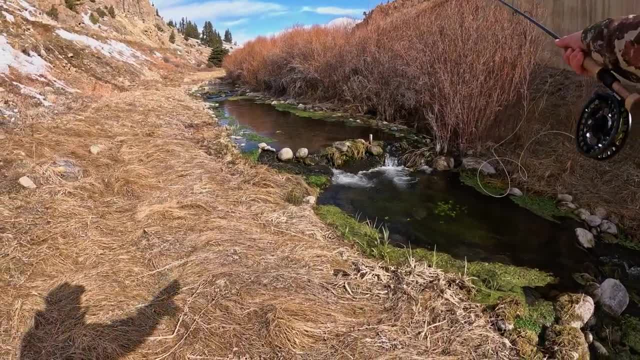 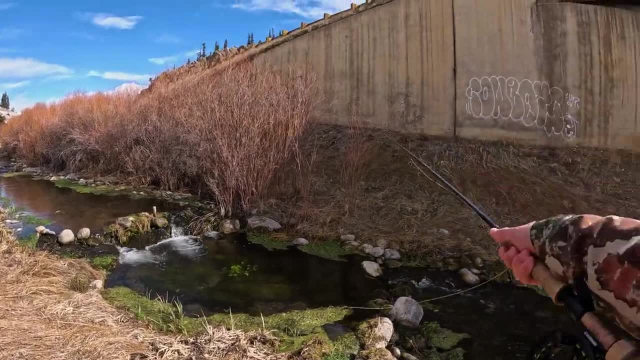 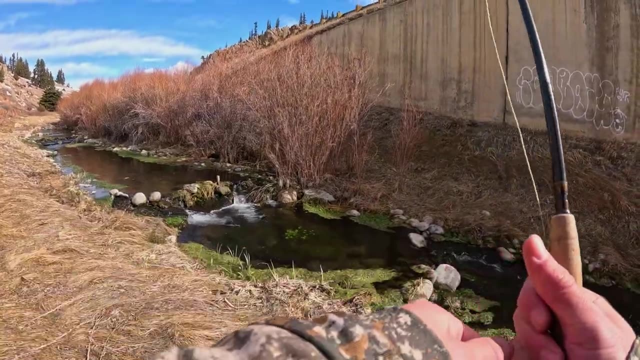 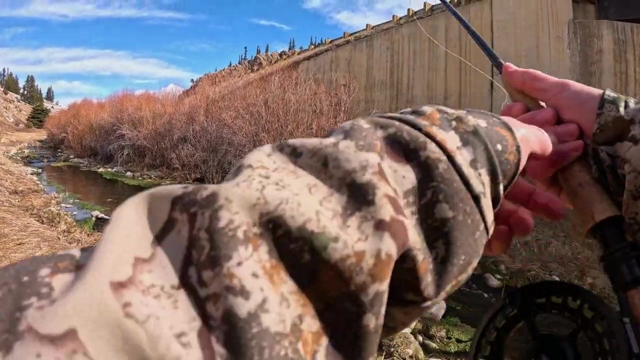 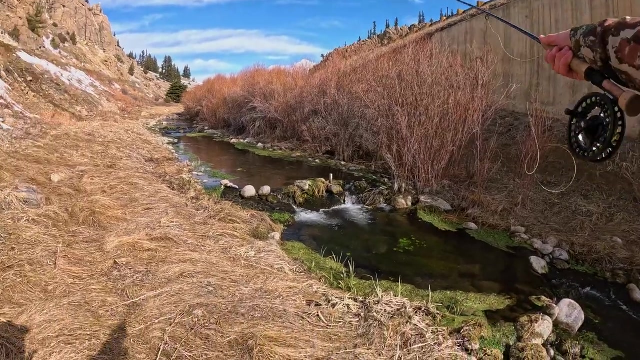 see him in there. oh all right guys. so he just broke me off. I don't know how the line snapped. I was probably already afraid he's still sitting there, so there's a chance. I just tied on one nymph so it might not break as quick, since there's less knots involved. let's see. 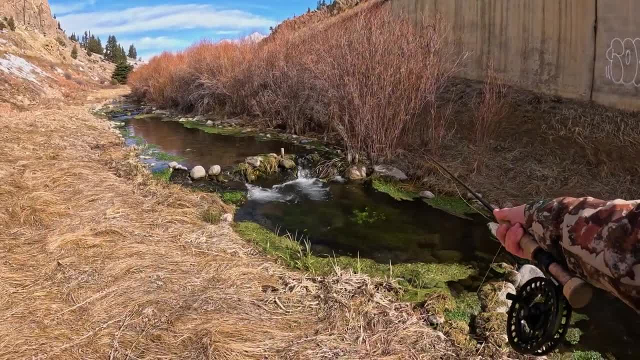 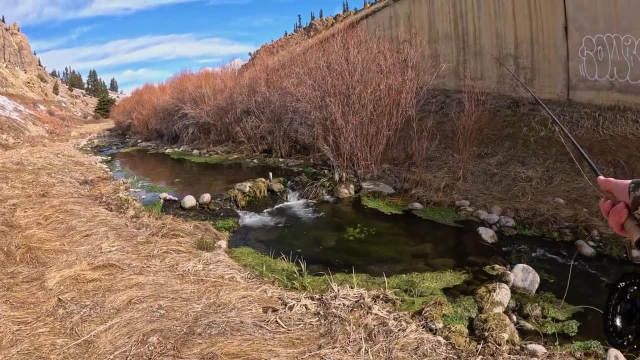 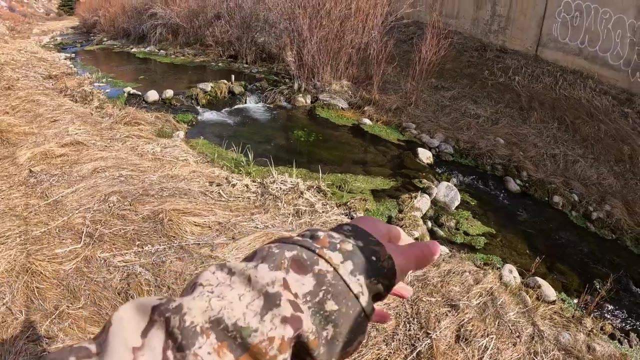 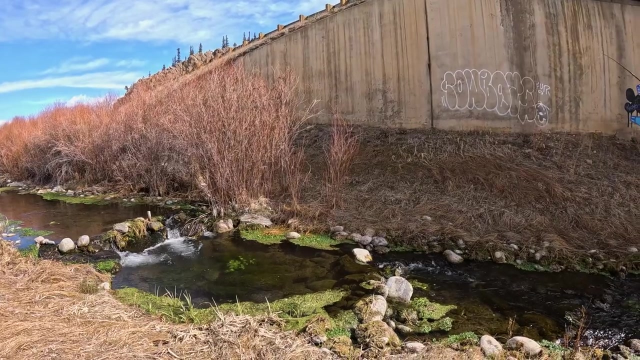 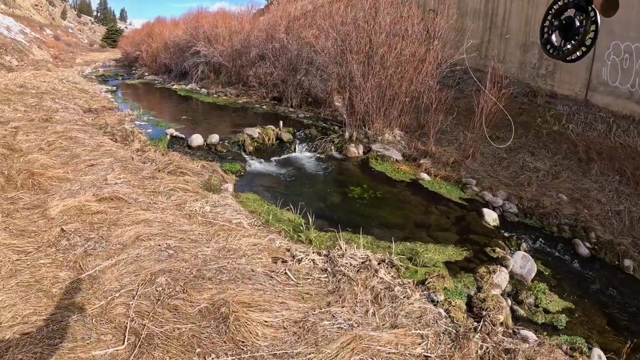 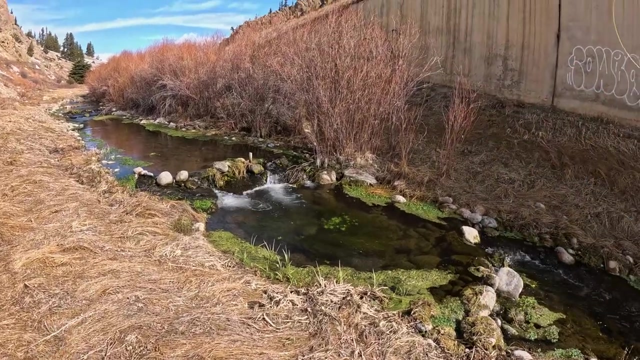 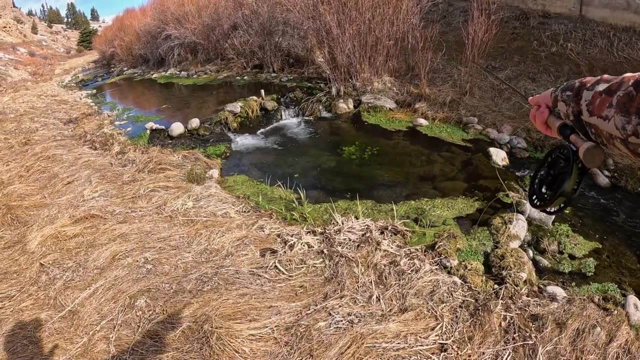 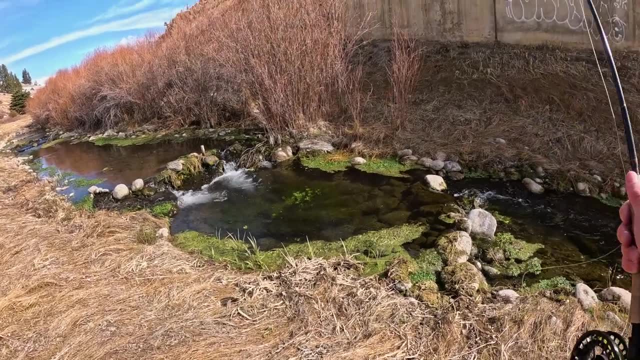 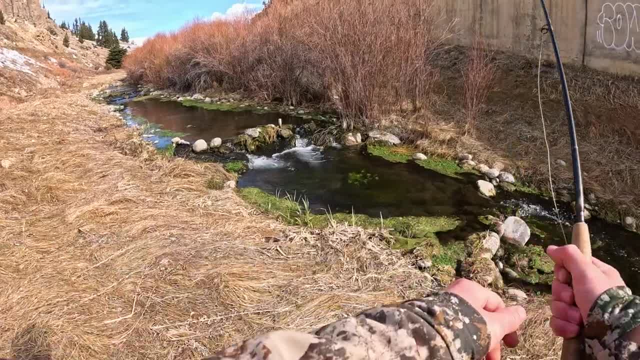 it might be tougher to sink in there, though didn't move, I guess I re-tied on a couple more nymphs trying to get them wet. actually, for us, let's see one, stop going for a second for me, let's see, guys, I'll try on something else again if this doesn't work well. 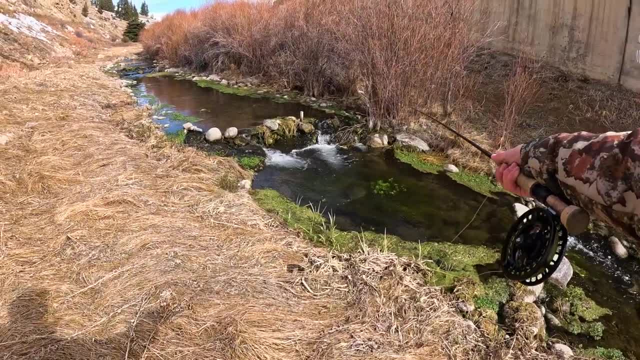 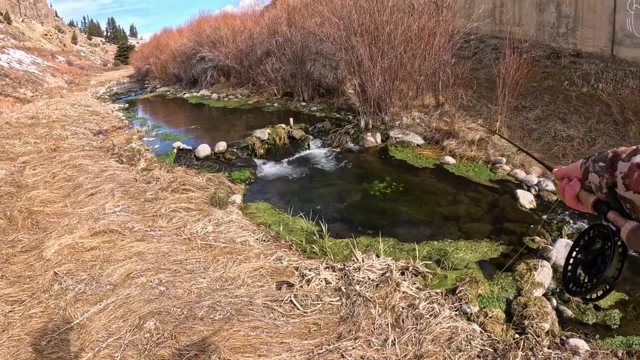 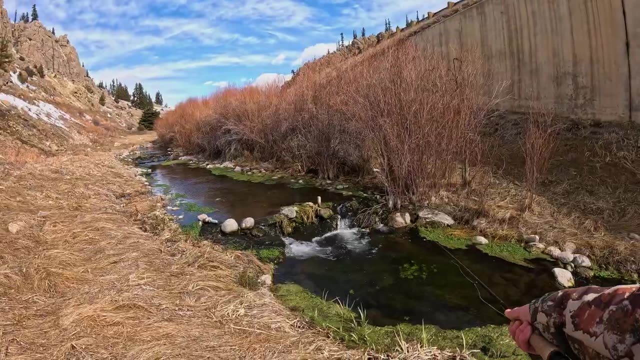 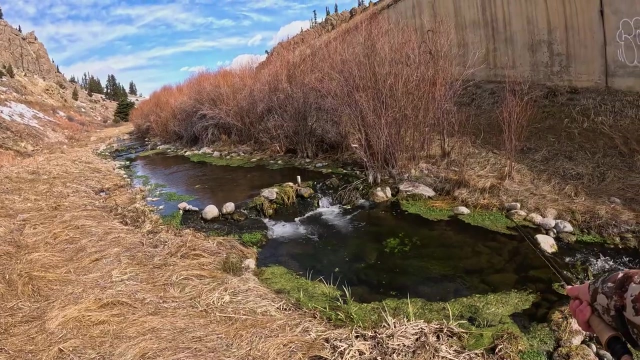 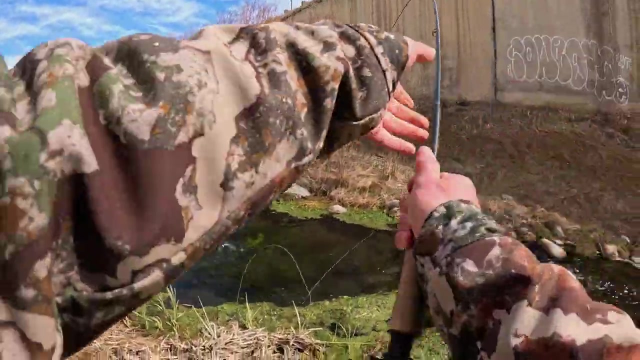 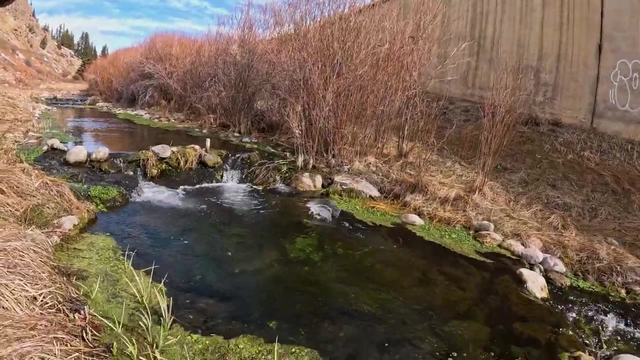 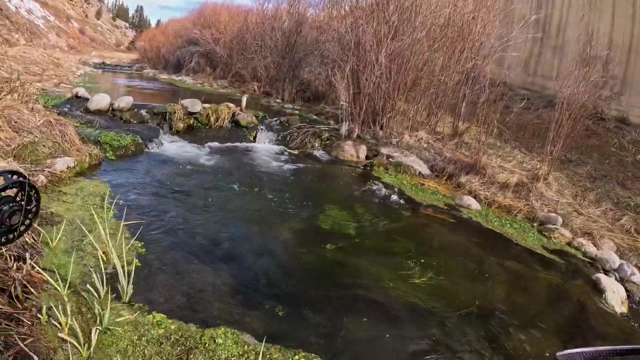 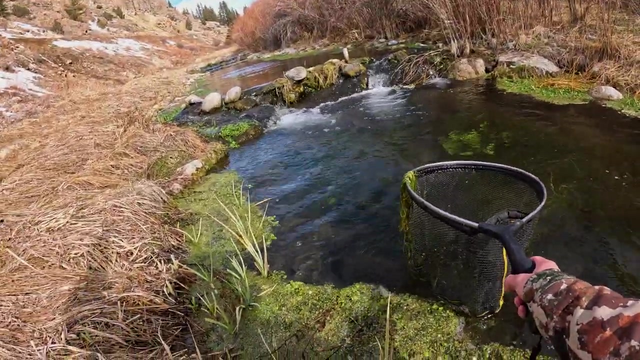 i have to come back another time time. for him it should be like tripping past it right there. he's just not even. oh, i see him, he's moving. oh, i got him. oh, it's a giant, he's a giant. look at him, look at that. 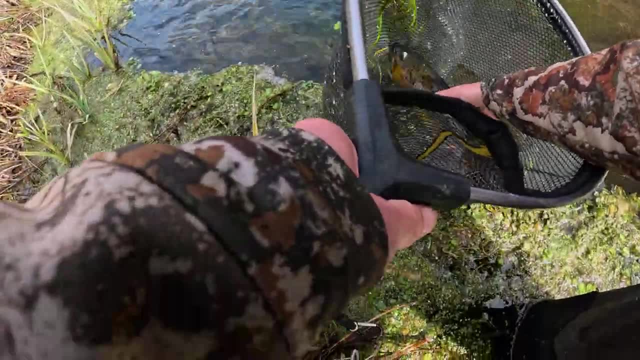 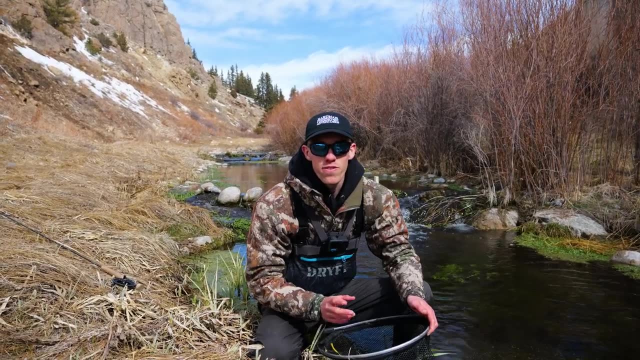 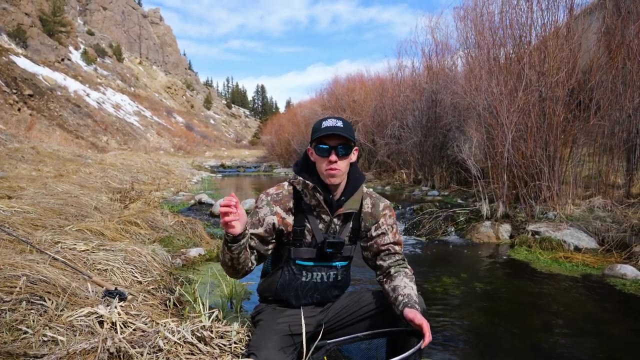 can't believe it. i'm recording. yes, i am the fish i was after. that's a big fish, all right guys. so i've switched flies about 50 times now and i finally- i didn't even think i had the fish on, i thought i was just on the bottom. i started pulling up. 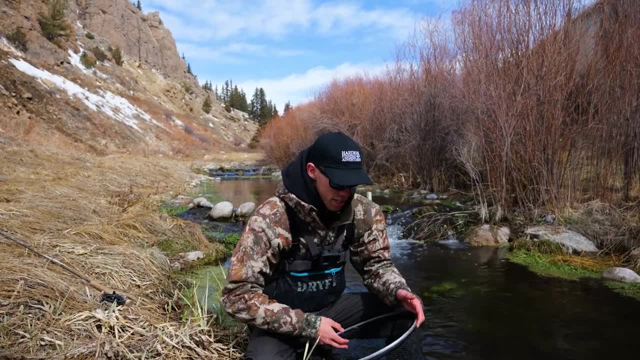 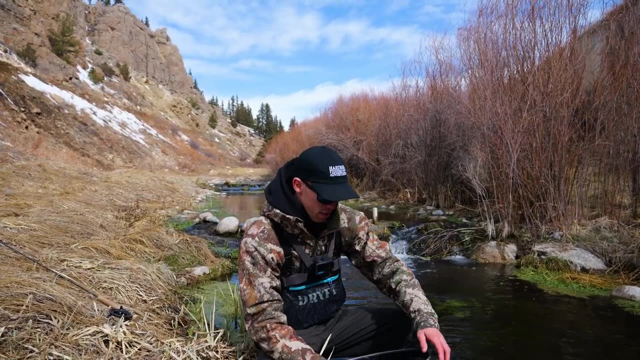 and then this guy's head starts shaking. but this is really big brown for this, like three foot wide spring creek. this hole he's in is actually a pretty big hole, but this is just a beautiful big brown shark here, so i'm going to go in and see if i can catch him. 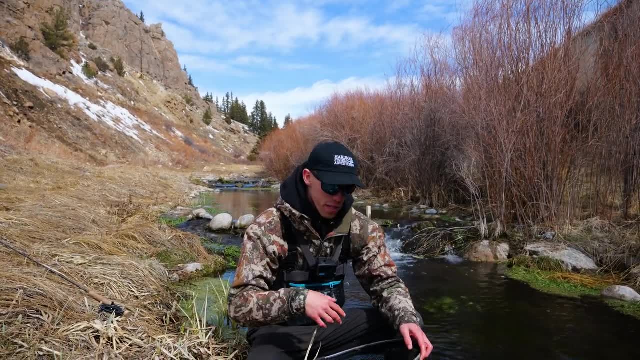 this is just a beautiful big brown shark here, so i'm going to go in and see if i can catch him. i'm just gonna hold them up briefly and then i'll get him back in the water, but this is an unbelievable fish for this size of creek here.